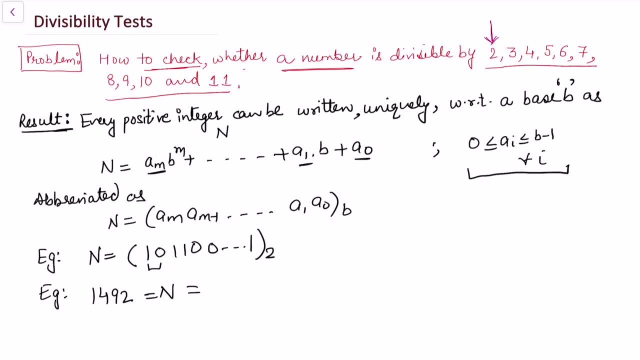 number, and I want to write this in terms of the base 10.. So for base 10, I will be using the same notation, because you see that if I want to write 1492 in this notation, so I will have 2, which. 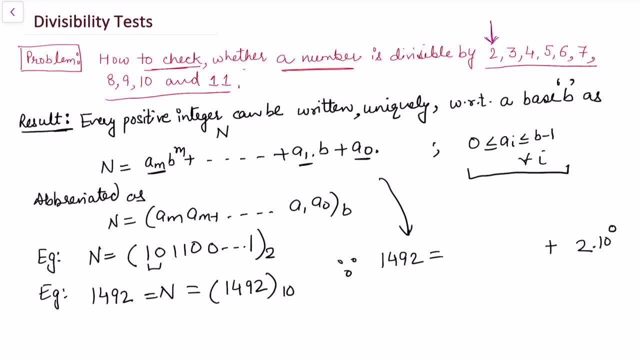 means 2 into 10, raised to power 0. So that is my A. A0 is B to the power 0. So I want to write B to the power 0 and then we can have 9 into 10 to the power, 1 plus 4 into 10, square plus 1 into 10. 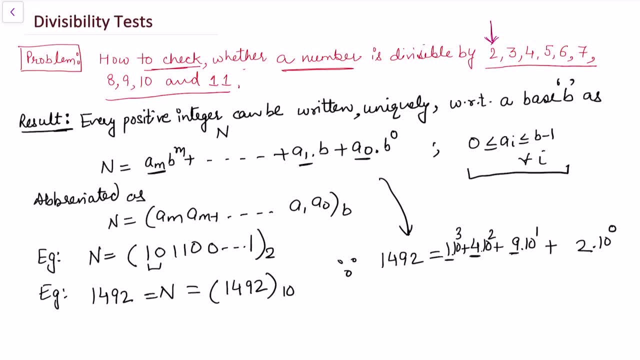 to the power 3.. So these are the coefficient 1,, 4,, 9,, 2, which are actually the values of AI, And so these AIs are appearing here and here. I'm writing this with respect to base 10.. And similarly we can. 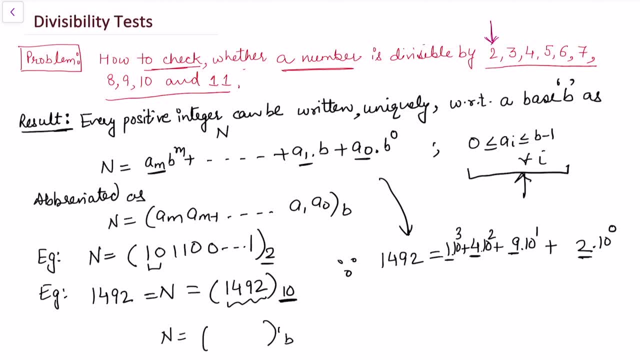 write the integers N with respect to any base B. Now, using the concept of writing any integer with respect to any base B, I will be using forward for my divisibility test. Now let's look at the first divisibility test, divisibility test for base 2.. And for this I'll be using this result. 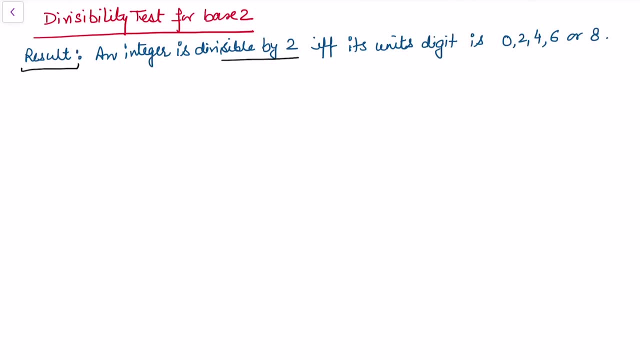 An integer is divisible by 2 if, and only if, its unit digit is 0,, 2,, 4,, 6 or 8, or we say that the number is even number. So to prove this result, let me to write an integer N. So this is: 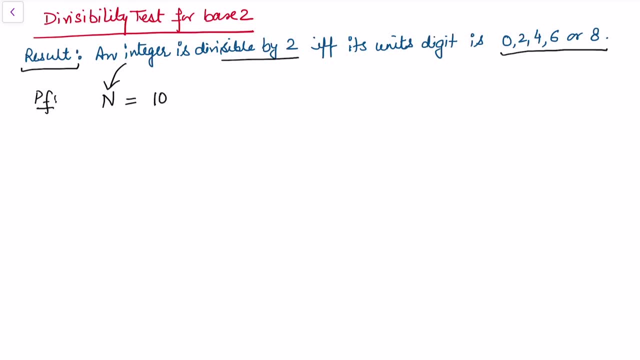 any integer into the decimal form. So here it is 10 raised to power M, into AM plus, and I can write AM minus 1, 10 to the power M minus 1 plus, so on A1 into 10 plus A naught. So let this be the representation of N with respect to base 10.. 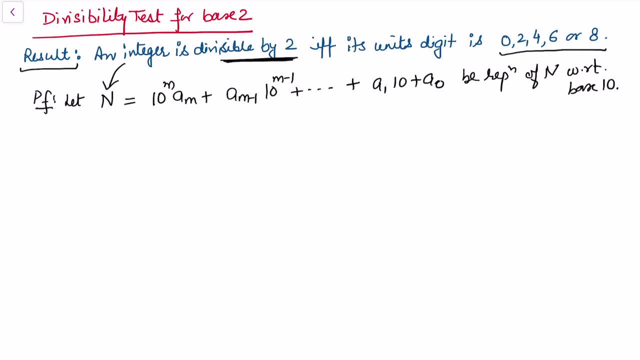 So once we know, with respect to base 10, and as we want to check the divisibility argument for the integer 2, so we notice that 10 this is congruent to 0 modulo 2, because 2 divides 10.. So we say that A is congruent to B modulo N whenever N divides A minus B. So this holds. 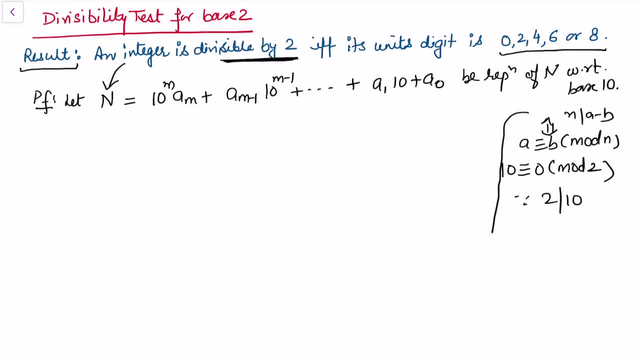 if, and only if, N divides A minus B. So with this argument, we saw that the 2, and obviously this means 10 squared, is divisible by 2 and 10 cube, and all the other powers are divisible by 2.. So, noticing these congruences, we can write down this: N integer. This is congruent to, since this: 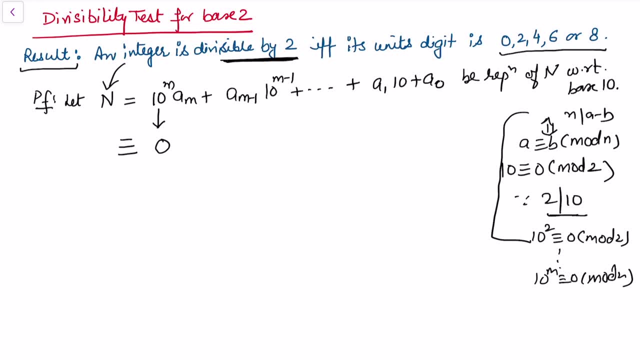 is 10 raised to power M, This is congruent to 0 modulo 2.. So replace this value by 0.. Similarly, this value is replaced by 0 and all other values will be replaced by 0, except the Last term, A naught, because this is not appearing- a multiple of 10.. This is with respect to: 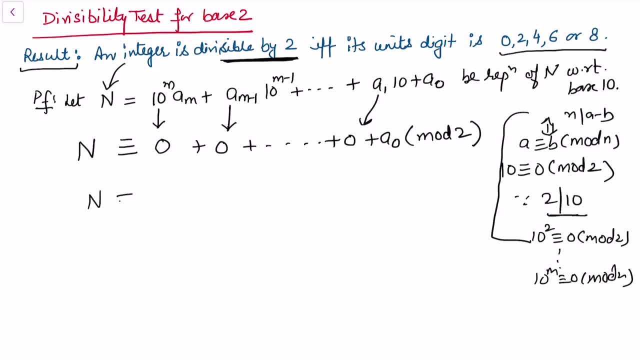 modulo 2.. So now we say that N is congruent to A naught modulo 2.. So we can say N is divisible by 2.. That means N should be congruent to 0 mod 2 if, and only if, A naught is congruent. 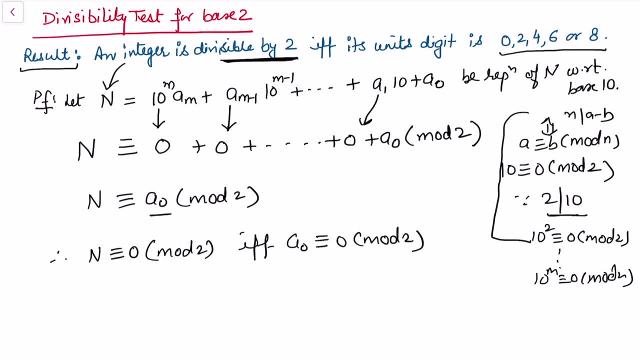 to 0 modulo 2.. So if A naught is divisible by 2 and A naught is congruent to N, so that will make sense that This number N is divisible by 2.. So to check this, this condition will hold. So we can say: 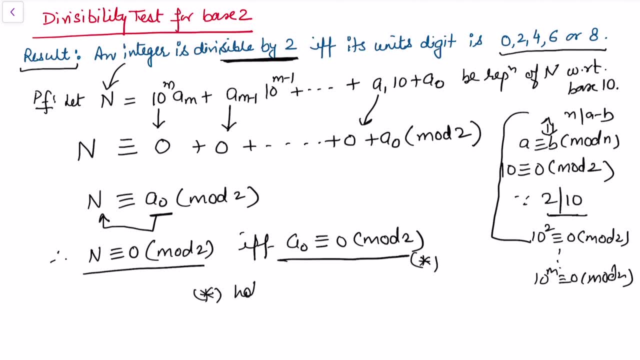 that star holds if, and only if, A naught can be either 0 or 2 or 4 or 6 or 8.. So because if you take any of these values to A naught, this will be divisible by 2, and hence N is divisible by 2.. 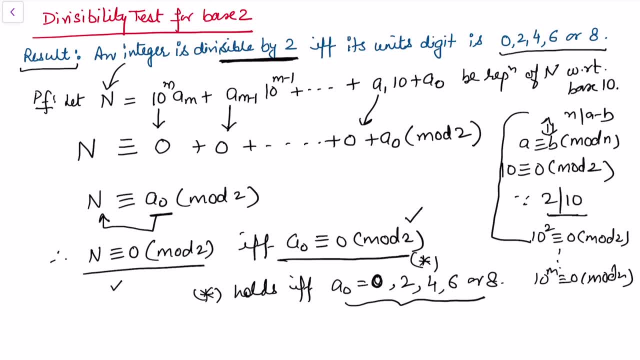 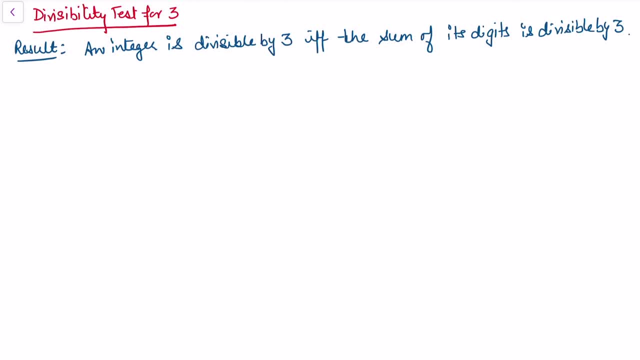 So we can say that an integer is divisible by 2 if, and only if, its unit digit is 0,, 2,, 4,, 6 or 8.. Now let's look at the result for divisibility test for 3.. An integer is divisible by 3 if: 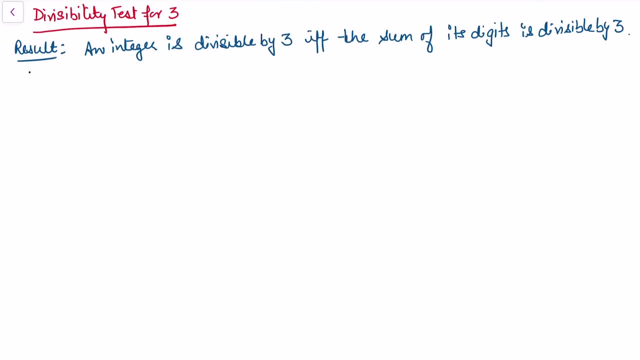 and only if the sum of its digit is divisible by 3.. Let's take an example first, before we prove. If I consider an integer- 1,, 5, 7, 1, 7,, 2,, 4. If I sum its digits, so sum digits. 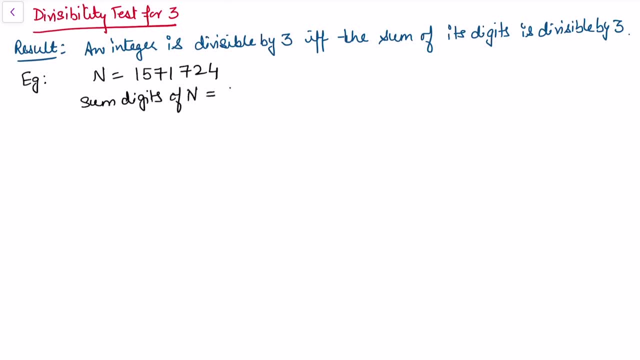 of this integer N, So we will get this as 1 plus 5 plus 7 plus 1 plus 7 plus 2 plus 4.. And the answer comes out to be 27.. And we know 3 divide 27.. So this means this number should be divisible by 3.. But why do we check this? Let's 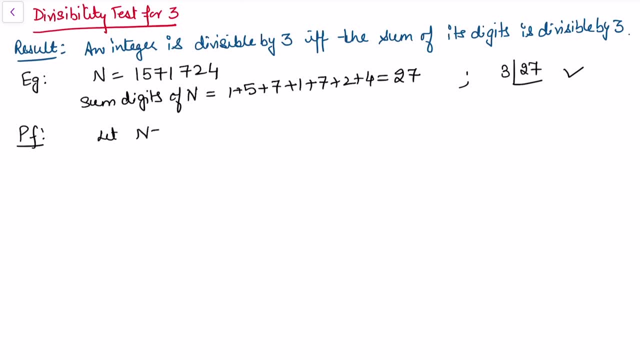 verify again: Writing N is equal to, again in the decimal form. So we get AM into 10 to the power M plus so on, plus A1, 10 to the power 1 plus A naught, And now notice that 10 is congruent to: 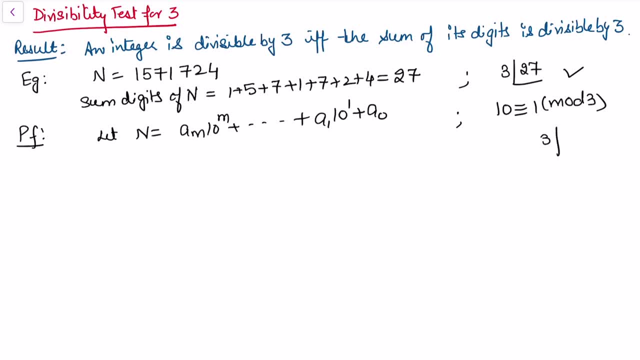 1 modulo 3.. Since 3 divide 10 minus 1,, that is 9.. So since 3 divide 9,, this congruence is true. If 10 is congruent to 1,, then that means 10 is congruent to 1.. So if 10 is congruent to 1,, 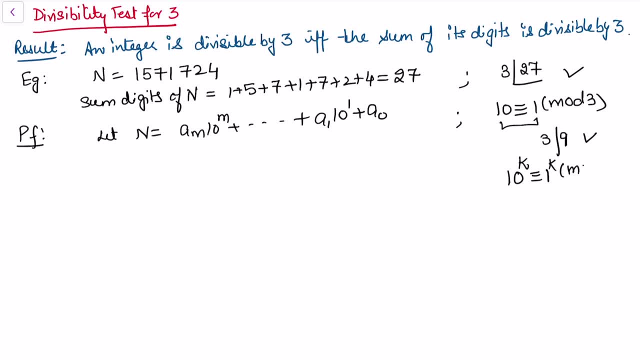 then 10 to the any power k is congruent to 1 to the power k modulo 3.. So now we do the replacement, This integer capital N. this is congruent to this. 10 to the power M. this particular is congruent to 1 raised to power M and AM will remain here and plus so on. 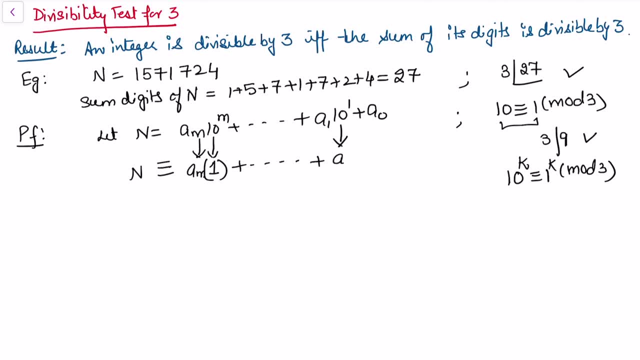 Similarly, this 10 will be congruent to 1.. So the remaining is only A1 into 1 plus A naught with respect to modulo 3.. So this is congruent to AM plus so on AM. And here we can see these are simply the sum of digits of the integer capital N. 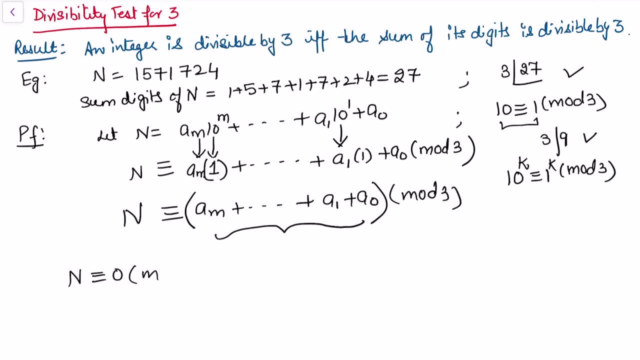 So we say that N is congruent to 0 modulo 3.. When I say 0 modulo 3, this means I am writing: 3 divides N, 3 divides N if, and only if. if this number is divisible by that means the sum should be. 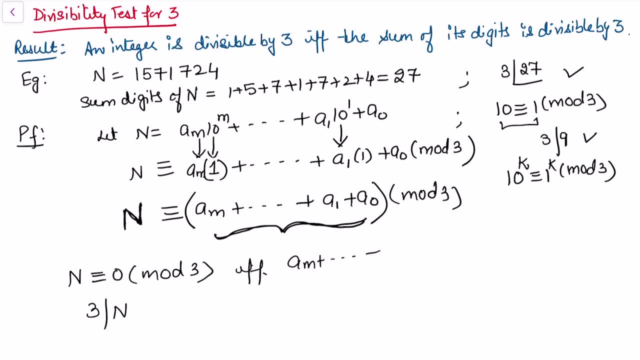 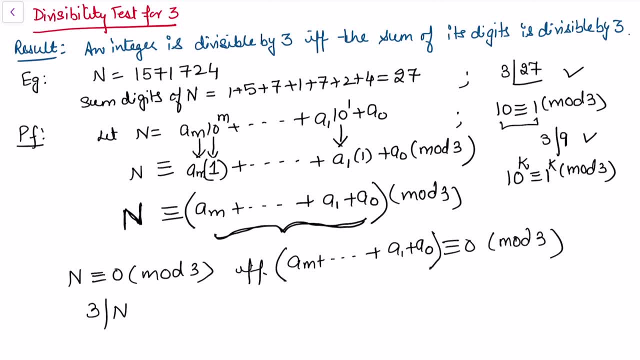 congruent to 0 modulo 3.. So this is congruent to 0 modulo 3.. So rather than checking on to the integer capital N, we check on to the digits of capital N. If this is divisible by 3, then we say: 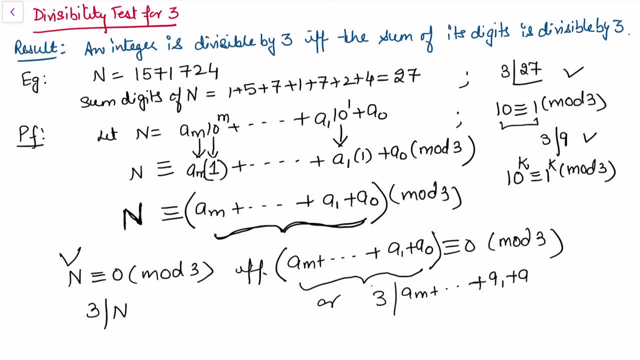 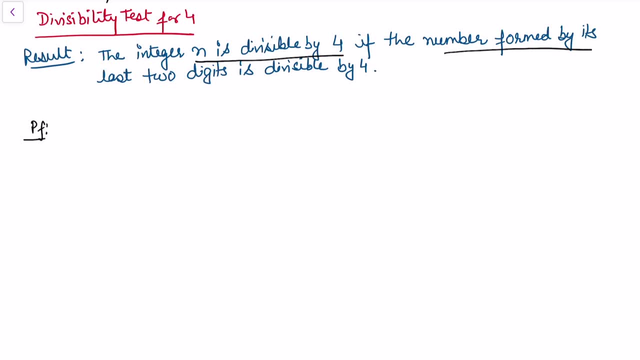 the original number that is divisible by 3.. Now divisibility test for 4.. So the integer N is divisible by 4 if the number formed by its last two digit is divisible by 4.. So let me to first give you an example. Let's consider an integer, capital N or small n. Here I have considered 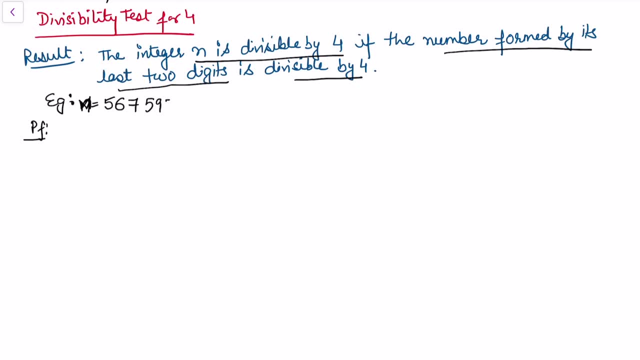 this is 5675972, and the last two digit are 72.. Since 4 divides 72,, so this particular number is divisible by 4.. So this is divisible by 4.. And now let's do the proof Again. for the proof, I want to: 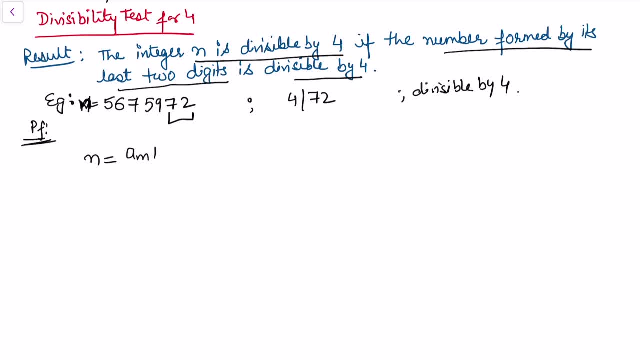 write the integer N into the decimal expansion. So this is AM into 10 to the power, M plus A1 into 10 plus A naught. Now I want to see when this 10 is congruent to modulo 4.. So if I take 10 is: 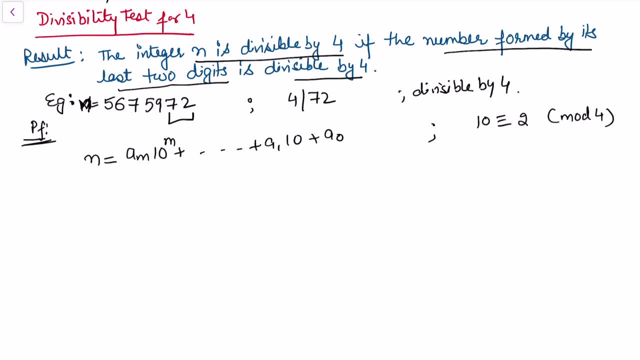 congruent to dash modulo 4, we know that 10 is congruent to 2 modulo 4.. And if I just square this term, 10 square, this is congruent to 2 square, that is, 4 modulo 4.. And we can see that 4 is. 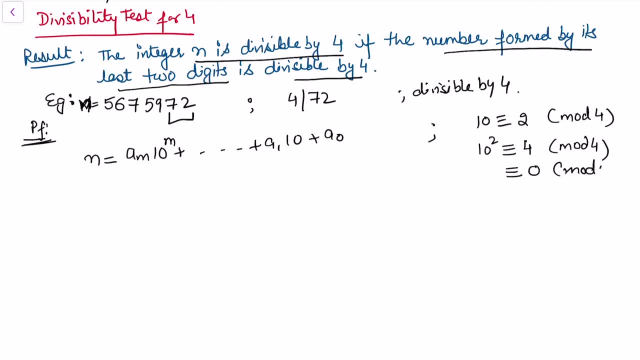 congruent to 0 modulo 4.. Because this particular 4, this one, is congruent to 0 modulo 4.. So this means 10 square is always congruent to 0.. And so now you can raise any power of 10 square. So if 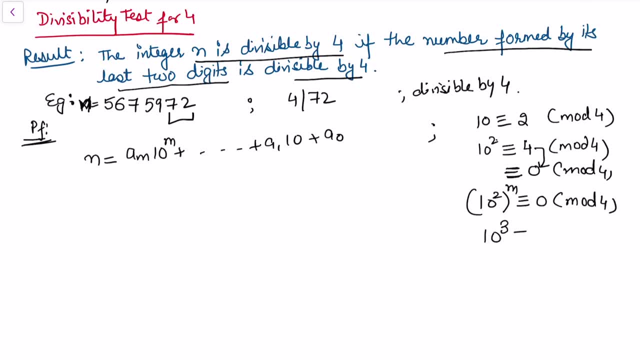 for the odd power say. for example, if I want to calculate 10 cube, 10 cube, we can write it as 10 square into 10 modulo 4. And 10 square is already congruent to 0.. So 0 into 10, this will also be. 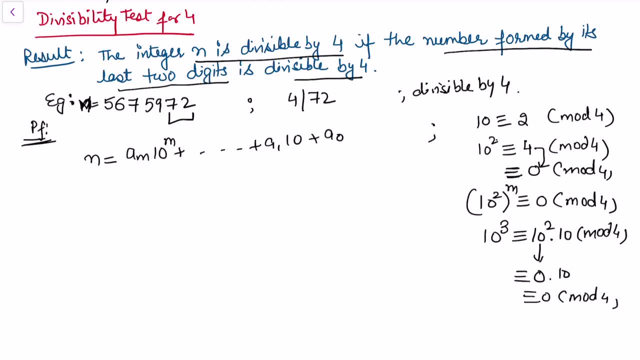 congruent to 0 modulo 4.. So all the power beyond this value, this will be always congruent to 0.. So this means N is congruent to this value is congruent to 0,. another value is congruent to 0. 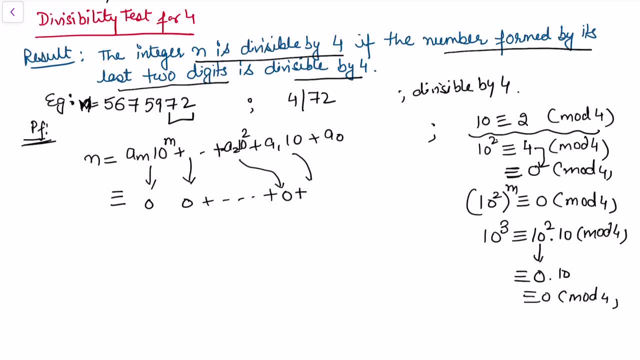 congruent to 0. The only remaining value is this one. Now, this value will remain as it is: A1 into 10 plus A0, because we said that 10 is congruent to 2 modulo 4. So this is congruent to A1 into 10. 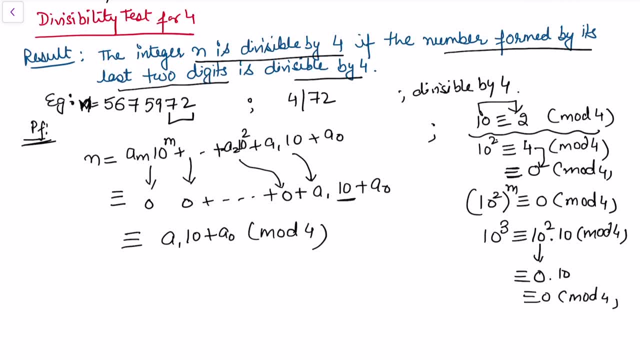 plus A0 modulo 4.. Now you can see that on one side we have integer N and another side we have last two digit. A1 into 10 plus A0 is actually the last two digit, Because if I want to write 72,. 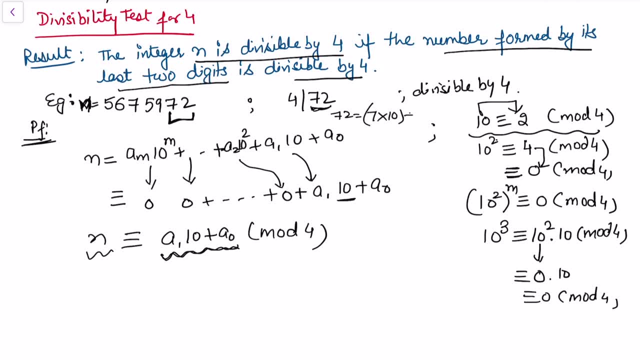 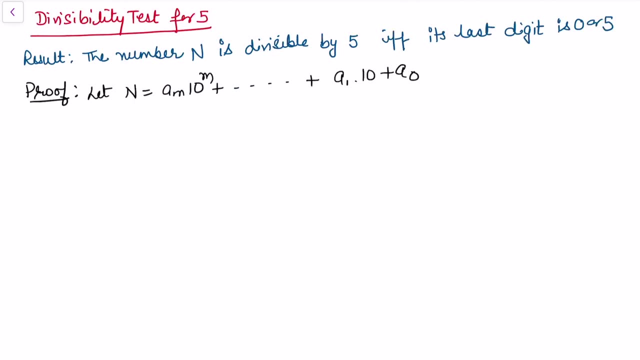 72 can be written as 7 into 10 plus 2.. So this expression is same as writing this form. So we say: 4 divide N if, and only if, 4 divide A1 into 10 plus A0, or 4 divide the last two digits. Now in divisibility test for 5, a number is divisible. 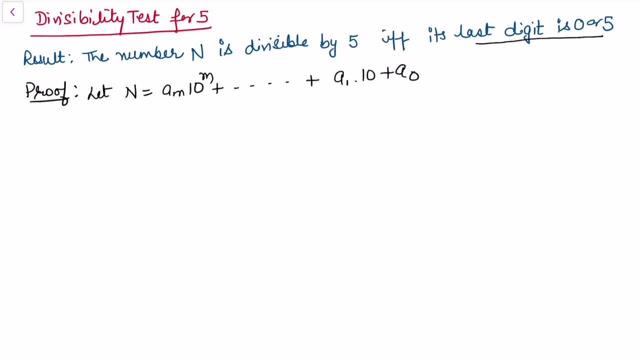 by 5 if, and only if, last digit is 0 and 5.. Again, writing N in terms of the decimal expansion, we know that 10 is congruent to 0 modulo 5, because 5 twos are 10.. So this means this: 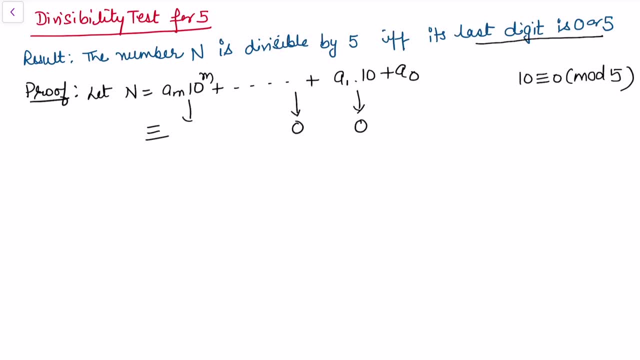 quantity is congruent to 0.. The next quantity is congruent to 0.. The next number here is congruent to 0.. All the numbers are congruent to 0, except that the last one, that is, A0, and then we write modulo 5.. So here we can see that N is. 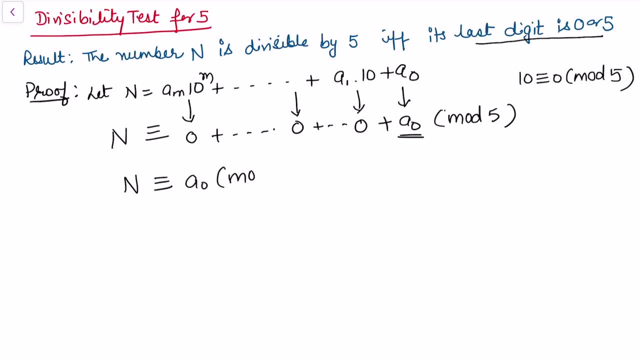 congruent to the last A0 modulo 5.. So from here it is very clear that 5 divides N if, and only if, 5 divides A0 and the choices for A0 can be either 0 or 5.. Now we discuss the divisibility test for. 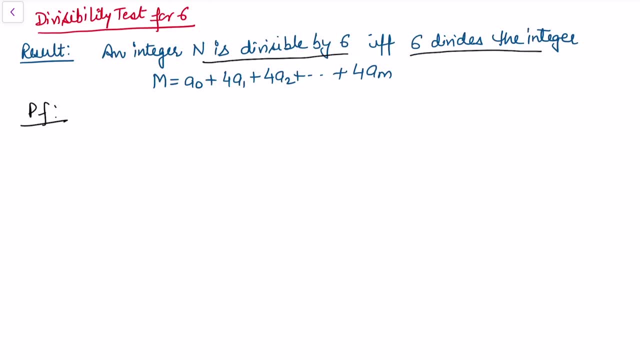 an integer N is divisible by 6 if, and only if, 6 divide the integer capital M, which is A0 plus 4 times the other integers, once the N has returned into the decimal expansion. So let capital N- and of course here you need to always keep in mind that N is written into the 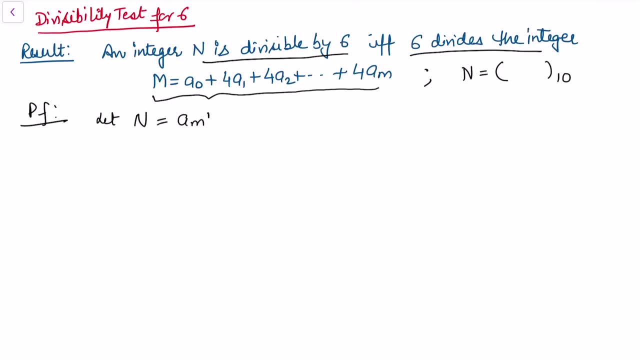 base 10.. So let's write N into the base 10.. So that is same expression that I have been writing again and again: A1 into 10 plus A0.. And also we notice that 10 is congruent to 4 modulo 6.. 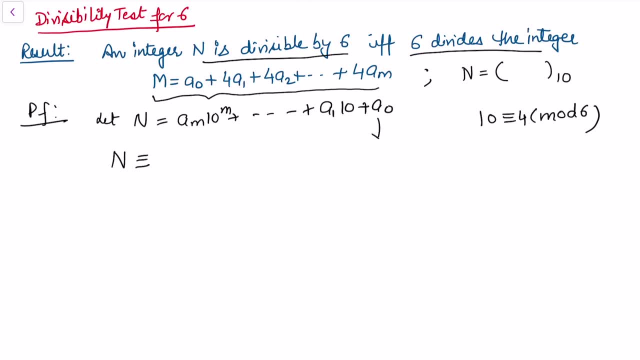 this means capital n. this is congruent to a naught, is as it is a naught, this particular will turn it to a1 into 4 and the other quantity, as you see that 10 raised to power square, this will become 4 square. this is congruent to 16. 16 is further congruent to 4 modulo 6. you can see that because 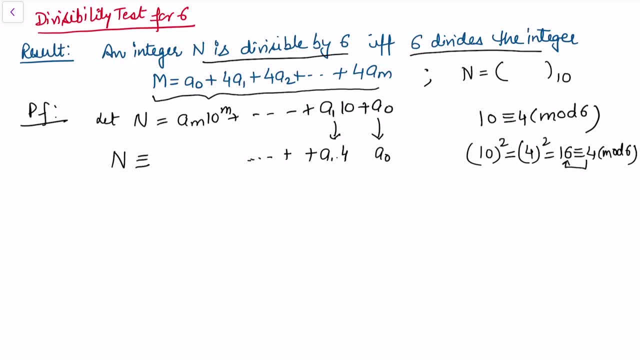 16 minus 4, this is 12. 6 divide 12. and similarly, if you take 10 cube, 10 cube which will raise the power of this quantity, so we can have 10 square into 10, 10 square is already congruent to 4 and 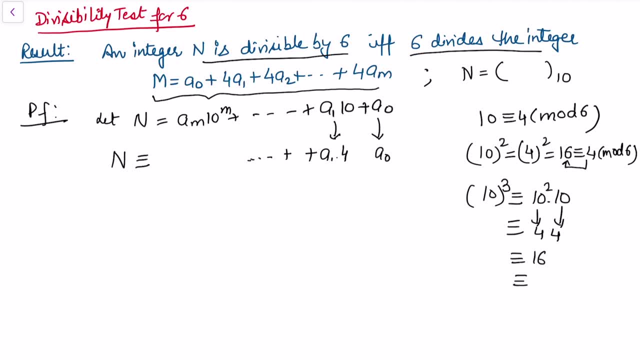 10 is also congruent to 4. so again you got 16, and again you got congruent to 4. so this way we can proceed and we know 10 to the power k will always be congruent to 4 modulo 6, so all. 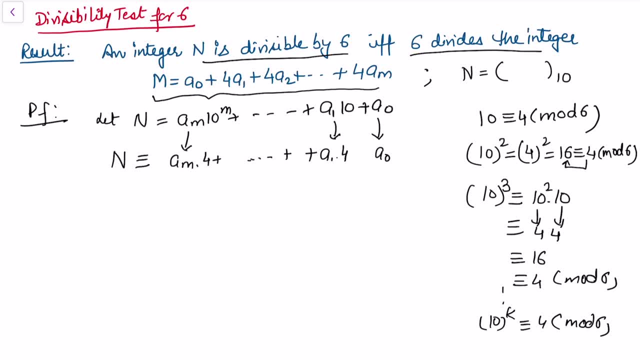 these expression are converted into 4 plus so on. so now you can see that here this is modulo with respect to c. so this expression writing a naught here and then 4 times the power of this quantity, so we can have 10, square into 4, and 10 is also congruent to 4. 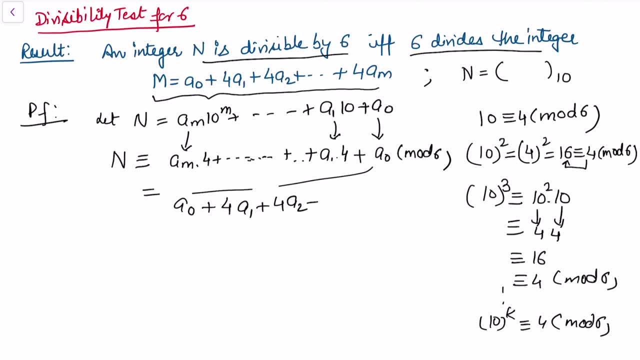 times a1, plus 4 times a2, plus, so on, plus 4 times a? m. this is the term with respect to modulo 6, so we can say that 6 divide n, if, and only if, 6 divide this particular integer, and which is a naught plus. 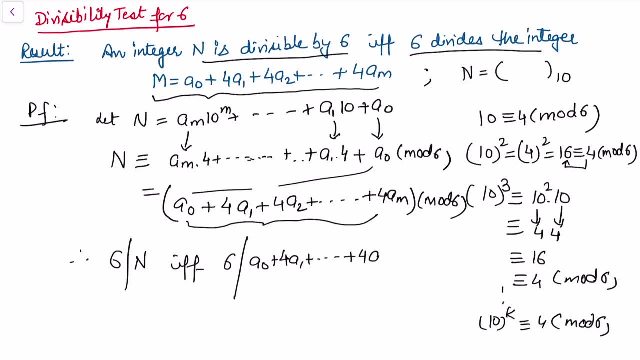 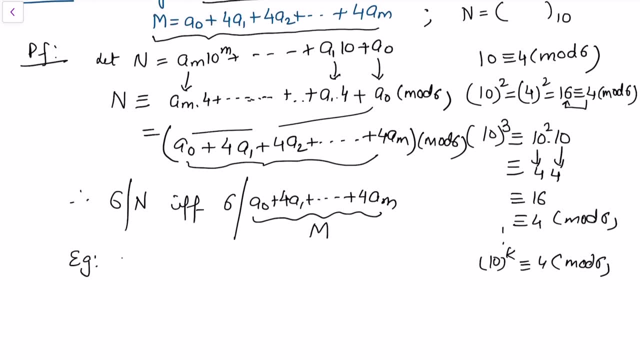 4 times a1, plus so on 4 times a, m, and this is what we have written as m. let's verify an example, very simple example. let me to consider capital n integer as 2, 1, 6. we know that 2- 16 is divisible by 6, but suppose, if i want to apply this test, 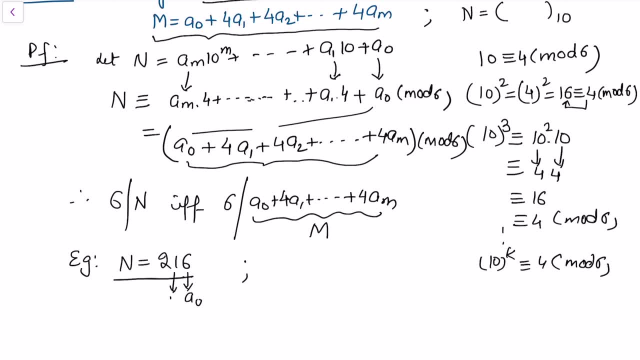 this particular 6 is a naught. this one is a1, this one is a2, because whenever we write n into the base 10, this is exactly the same digits. so we apply here a naught. that is 6 plus 4 times a1, which is 1, plus 4 times a2, which is 2. so this is 6 plus 4 plus 8. 6 plus 4 is 10 plus. 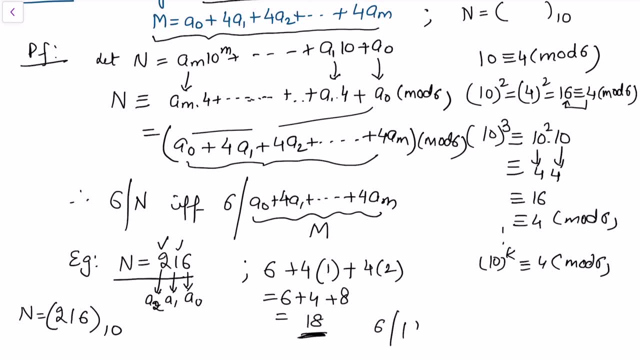 8, 18. now we know that 6 divide 18. if 6 divide 18, 6 will definitely divide this integer n and hence, to check that 6 divide n, we must need to divide 6, divide a naught, the last digit plus 4 times all. 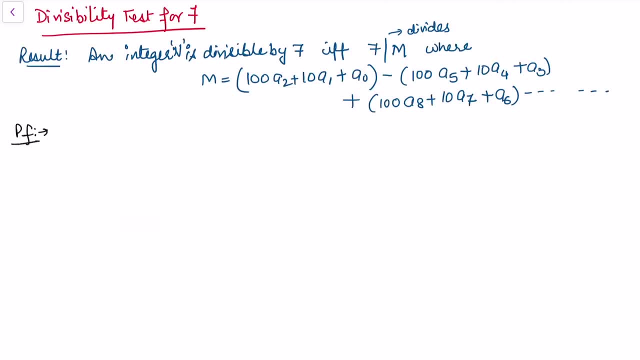 other digit, their summation should be divisible by 6 in the divisibility test for 7 and integer n is divisible by 7 if, and only if, 7 divides m, and where m is 100 times a2 plus 10 times a1 plus a. 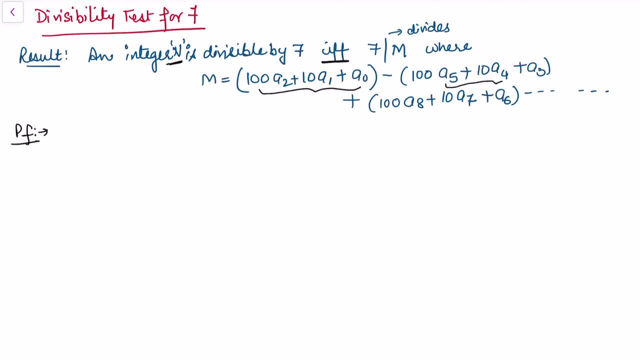 naught, and then same thing. we repeat for the next digits, as you can see that, for 3, 4, 5, and then for 6, 7, 8, and we keep on repeating. now let's see how we have done this. n is a m into 10 to the power m plus a m minus 1. 10 to the power m minus 1 plus. 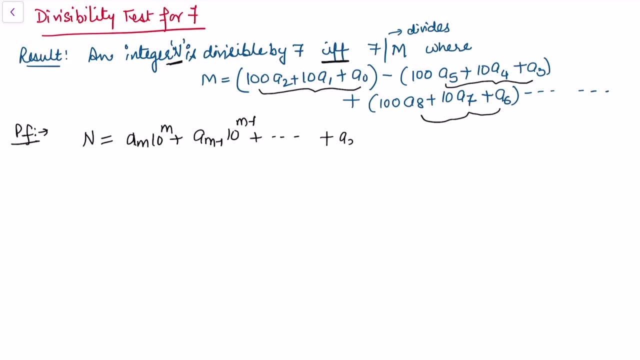 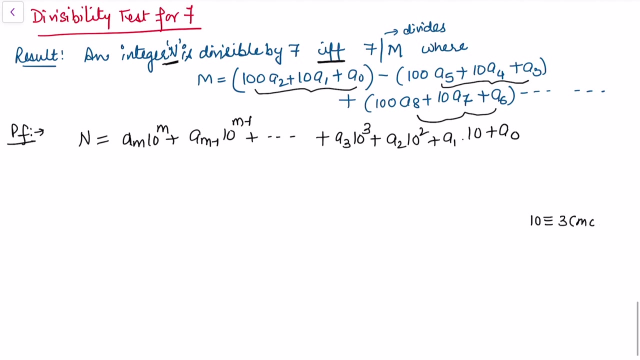 so on. and let's write a 3 into 10 cube plus a square, 10 square plus a 1 into 10 plus a naught. now notice that i want to calculate with respect to modulus 7. so 10 is congruent to 3 modulo 7, and then we can calculate 10 square. this is congruent to 9, 9 is congruent. 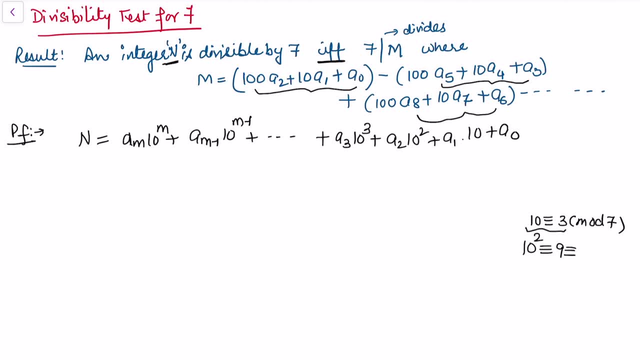 to, because if i just simply take the square of the previous term here, so 9 is congruent to 2 modulo 7, and then i take 10 cube. 10 cube is 1000 and this quantity is congruent to minus 1 modulo. 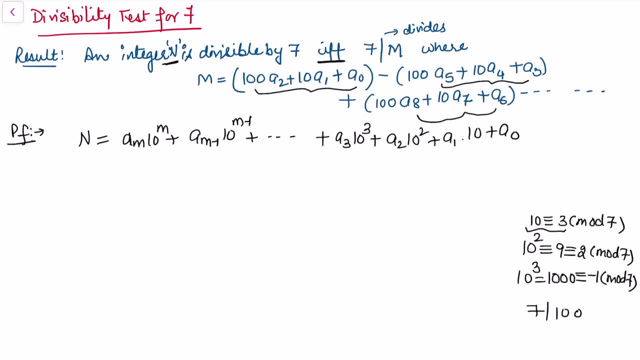 7, because 7 divide 1, 0, 0, 1, it divides this quantity. so now, if i, if i just try to replace this quantity, this is congruent to so see, this a naught will remain as a naught, this 10 will remain. 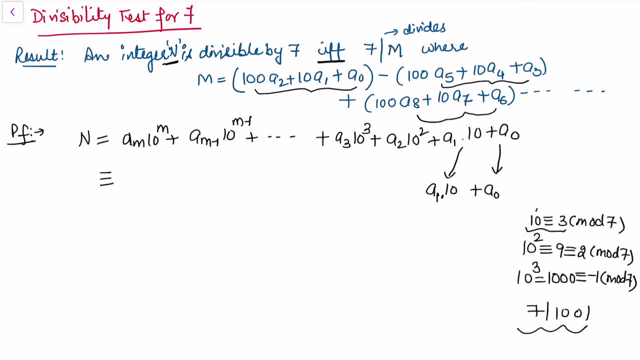 as it is a 1 into 10, or we can at least reduce it to 3, that is fine, but 10 square, 10 square. we can see this is also congruent to 2. it's not further replaced in the formula. i've kept it as 100 only. 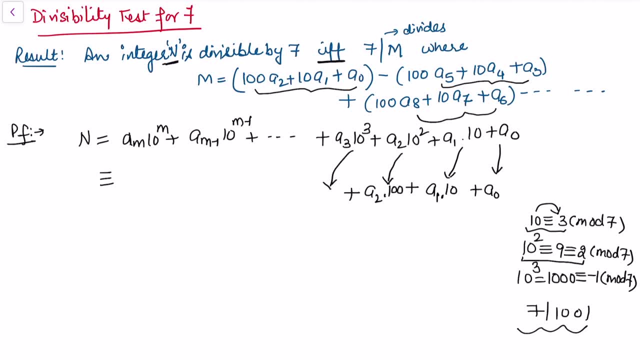 so keep it as 100 plus 10 cube. now this quantity cube. this is congruent to minus 1. so once it's congruent to minus 1, we replace it as minus a3, and then the next quantity would be a4 into 10 to. 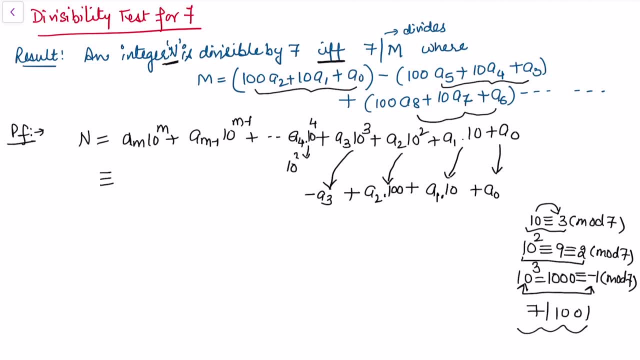 the power 4. now this 10 to the power 4 is having 10 cube into 10. so this 10 cube will give me a minus sign and a4 into 10 will remain as it is with a minus sign. similarly, now the next a5 will. 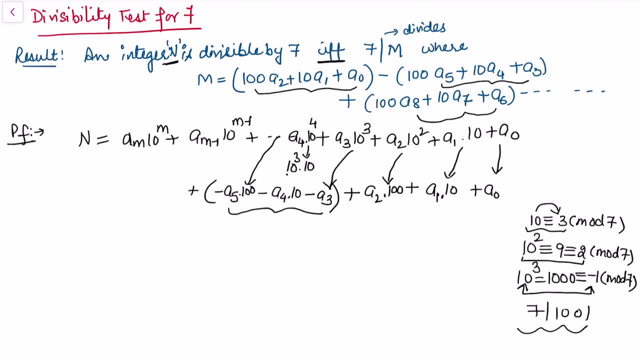 give me minus a5 into 100 plus, so on, and noticing that here we have taken 10 to the power, 1 outside and 10 cube. so if this power is an odd, we'll always get a minus 1, if this power is even, we'll. 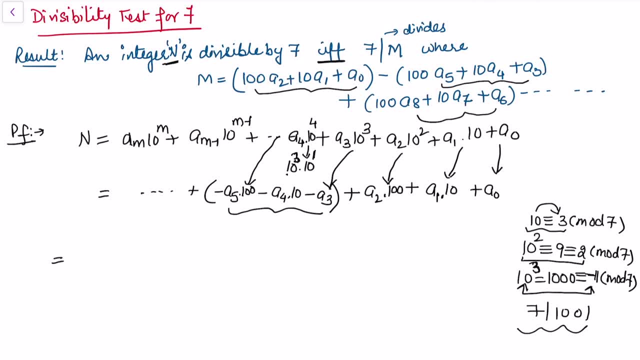 get a plus 1. so let me to explore it further. one more step we will see now: 10 to the power, a6 into 10 to the power, 6 plus a7 into 10 to the power 7 plus a8 into 10 to the power, 8, suppose, if i want. 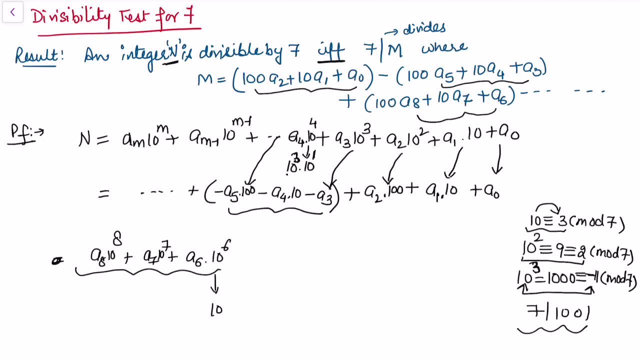 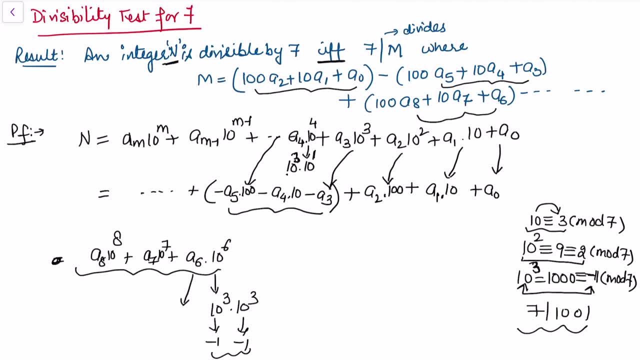 so both will turn into plus 1, so this quantity remain only a6. similarly, this quantity will remain only a7 into 10. this quantity will remain only a8 into 100. and so this, this three terms, comes with a plus sign. and now you can notice here: one time we have a minus sign, then we have 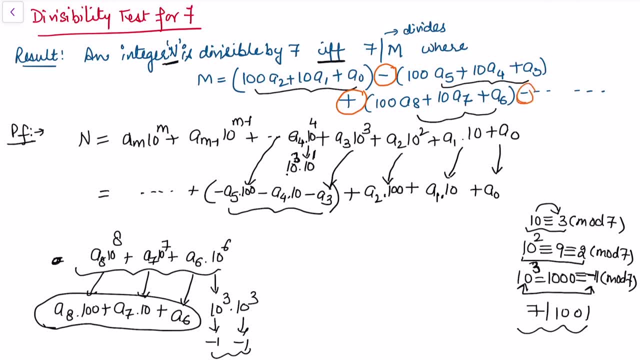 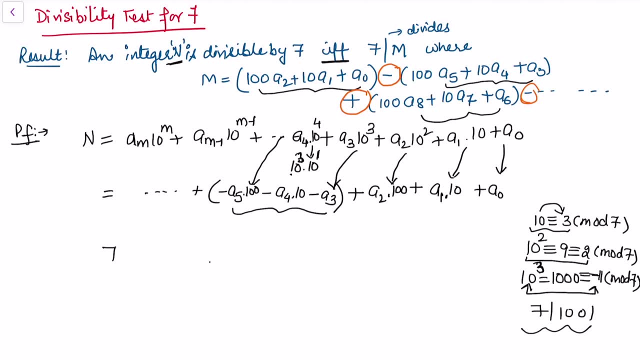 a plus sign. so, alternatively, it will keep on going and hence we get our result that the number, this capital n, is divisible by 7 if, and only if, 7 divides m, where this m is taking three tuples, taking three digits together, a0 plus 10 times a1, plus 100 times a2, and then subtract this will become a3 plus. 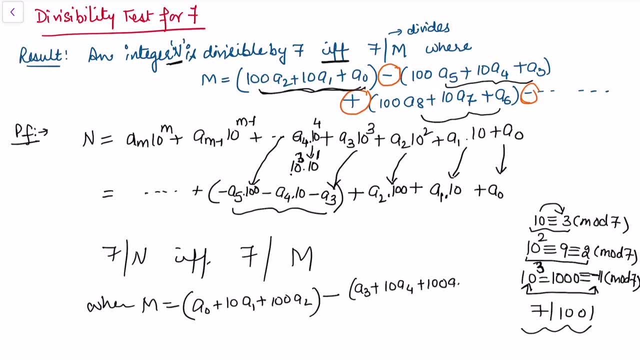 10 times a4 plus 100 times a5. then add: we get a6 plus 10 times a7 plus 100 times a8. then subtract: we get a9 plus 10 times a10 plus 100 times a11 plus so on. so it depends upon how many digits were there in our original integer and the sequence we 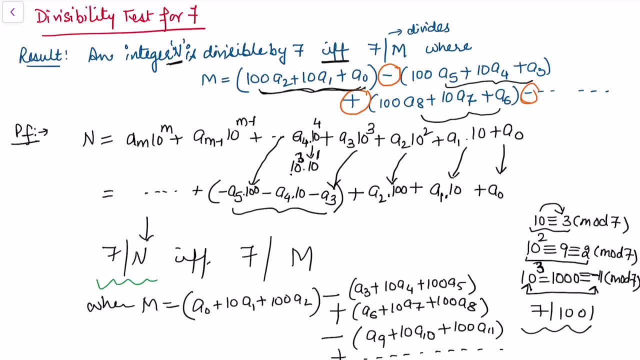 will follow if we want to divide a number by 7. that is why this divisibility test for 7 is not in very common. because of this term that we have to divide by 7, because of this term that we have to take alternate negative, positive, and then we have to multiply the 10 certain power. but now 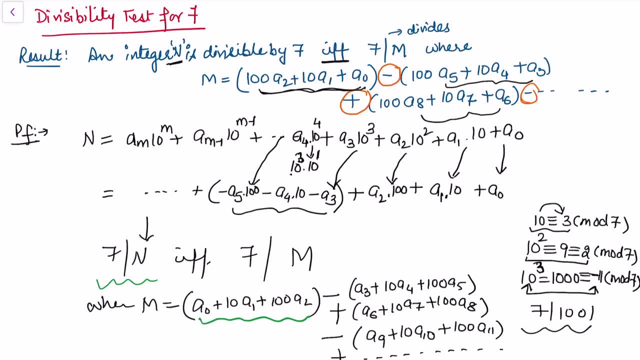 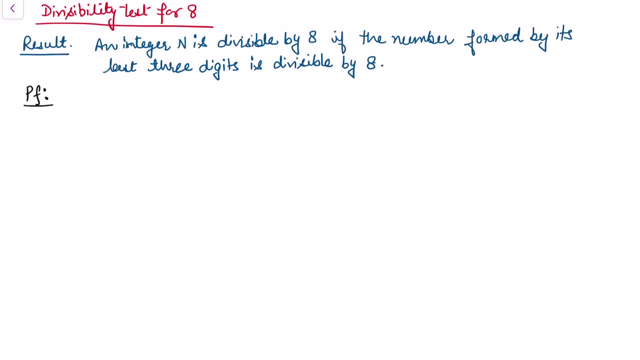 interestingly, we know from the congruences that there is a divisibility test available for the integer 7 also. so now we'll be looking the divisibility test for 8, and it is quite identical as we did for the integer 4. so an integer n is divisible by 8 if, and only if, the numbers formed 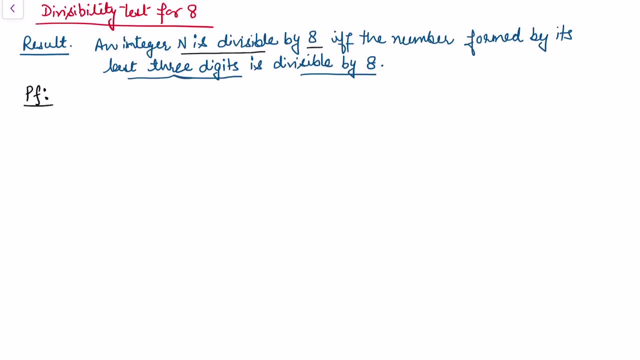 by its last three digit, is divisible by 8.. so let's take an example first. and if i consider an example, we see that 5, 6, 7, 5, 9, 7, 2- this number was divisible by 4. so i'll write: this: is divisible by 4 as 4 divide 72, and 72 was the last digit. this number is not. 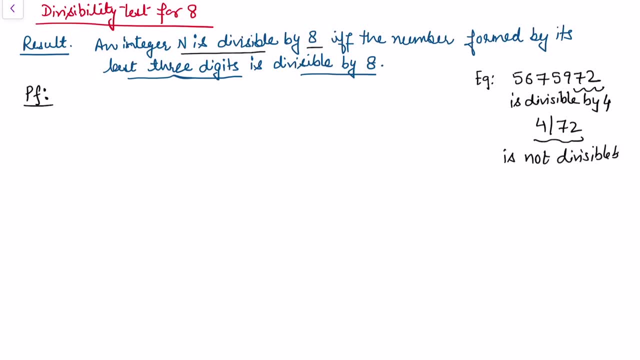 divisible by 8. this is not divisible by 8, because the last three digit for 972 is not divisible by 8. so now let's take an example. so that means it's not that every number which is divisible by 4 is also divisible by 8.. so now let's take another example, and here i'm 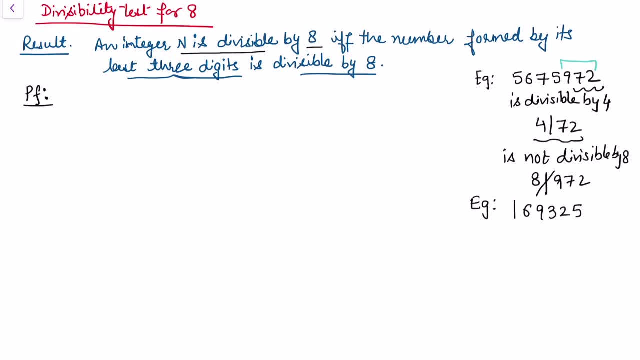 considering 1, 6, 9, 3, 2, 5, 94.. now, this number is also neither divisible by 4, nor it is divisible by 8. but let's consider one more example, and here i might want to consider 3, 2, 5, 8, 9, 1, 0, 4. 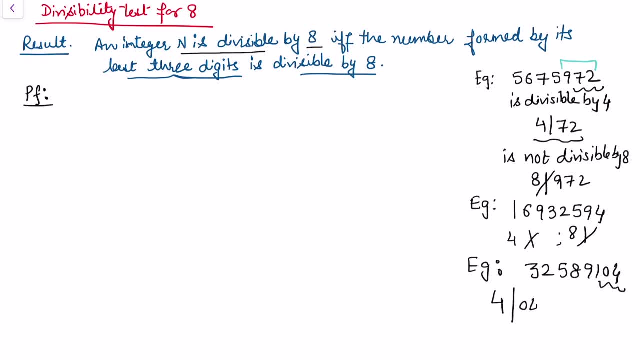 now you can see that 4 divide the last two digit, 0, 4, so this number is divisible by 4 and the last three digit, which is 104. they are also divisible by 8, so this number is divisible by both 4 and 8. 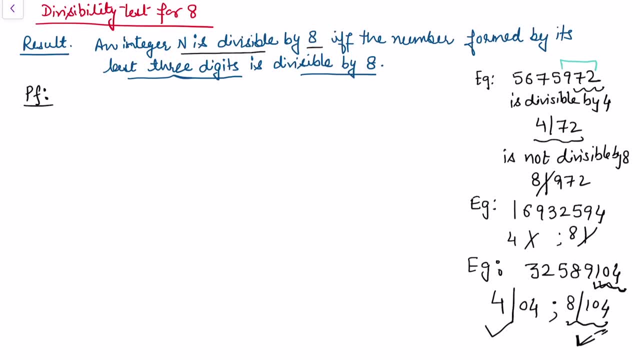 so we need to verify always: what number are we searching. if we are searching for the number which is divisible by 8, we should always focused on to last three digits, and the proof is also very similar, as we are already doing for the other cases. let n be written in. 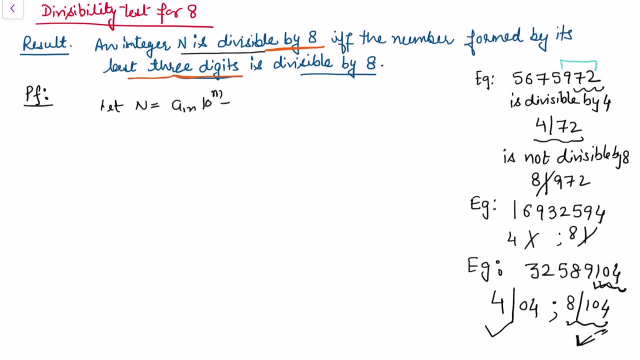 to the decimal form. so here we have a m, 10 to the power, m plus so on, plus a, 1 into 10 plus a naught, and as we have noticed that 10 is congruent to 2 modulo 4.. we have seen the 10 cube. this comes out: 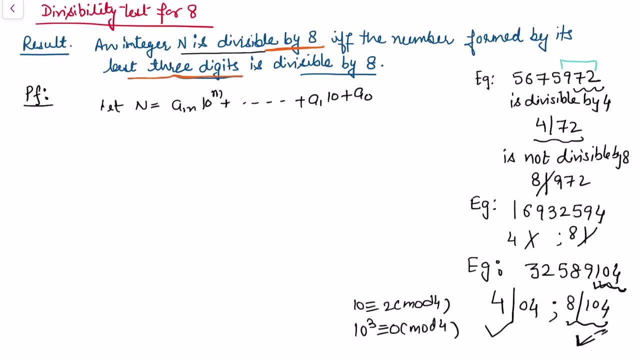 to be congruent to 0 modulo 4.. so we will follow the same procedure for 8 as well, and we notice that 10 is congruent to 2 modulo 8.. now let's raise some power, so we get 10 square. this is: 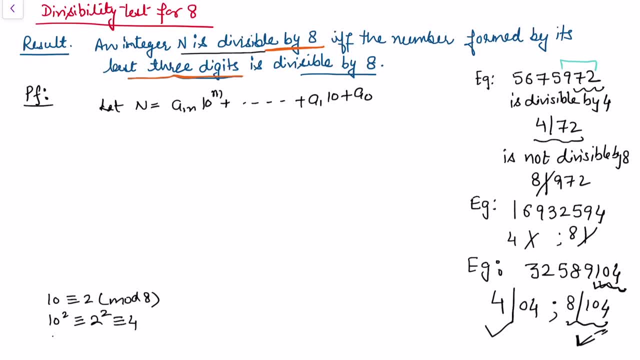 congruent to 2 square, which is congruent to 4, and we will follow the same procedure for 8 as well. let's raise one more, 10, so 10 cube. this is congruent to 2, to the power 3, that is, 8 is. 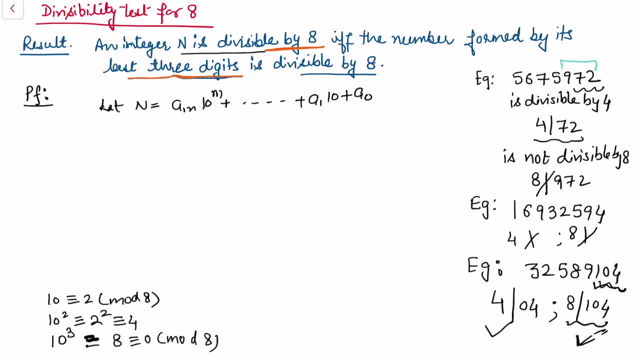 congruent to 0 modulo 8.. so this means 10 to the power, 3 is always going to be 0, and so the higher other values. so here we can say that n is congruent to a m, 10 to the power, m plus. so on, plus a 3, 10. 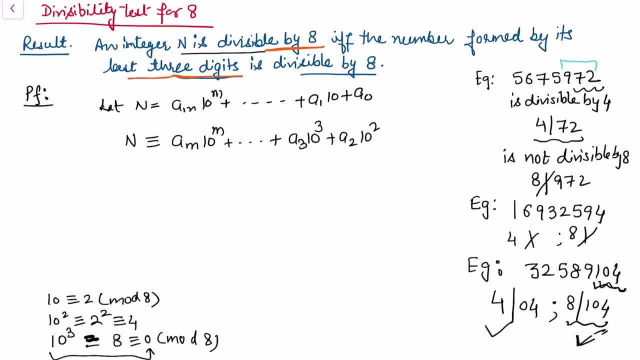 to the power 3 plus a 2, 10 square plus a 1 into 10 plus a naught. this is the value for n. this is further congruent to of these quantities congruent to 0, except the last terms. so this is a 2 into 10 square plus a 1 into. 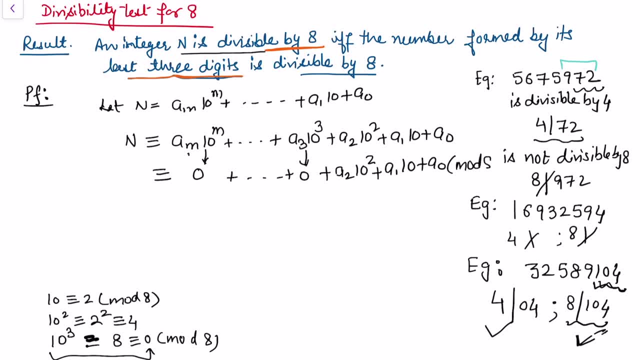 10 plus a naught, modulo 8.. so 8 divides n if, and only if, 8 divide this value, m, where m? this is a 2 into 10 square plus a 1 into 10 plus a naught, and if i look this one together, these are the last. 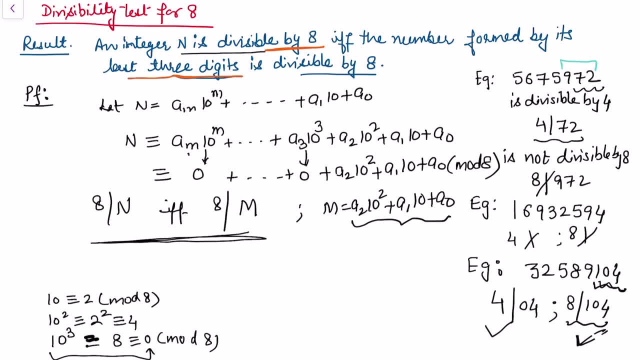 three digits. so if 8 divided by n is congruent to 0 modulo 8.. so if 8 divided by m is congruent to 0 modulo 8.. so if 8 divided by last three digit, 8 will divide the integer capital n. now in the 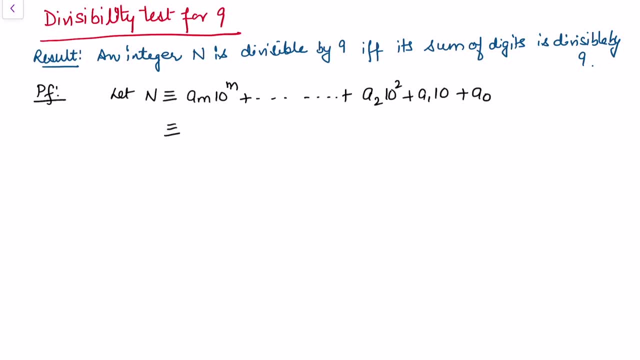 divisibility test for 9, and integer n is divisible by 9 if, and only if, its sum of the digit is divisible by 9.. so this is very much similar to the one we have done for the divisibility test for 3, and noticing that 10 is congruent to 1 modulo 9.. so let's replace 10 by 1 wherever we have 10. 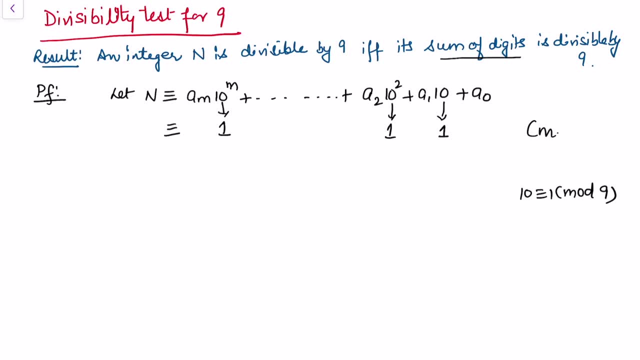 let's put this into the congruent 1 with respect to moduli 9.. so other digits will follow as it is. so this is a1 into 1, this is a2 into 1, plus so on am into 1.. so n is congruent to sum of digit am. 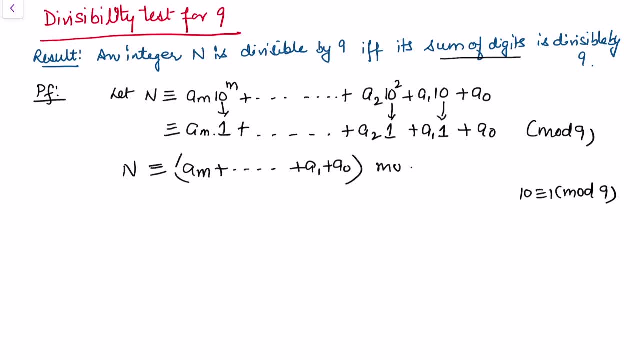 a1 plus a naught, moduli 9. so we can say that 9 divide n if, and only if, 9 divide this sum of the digit am up till a naught, and hence the result follows for the test for the nine, for the 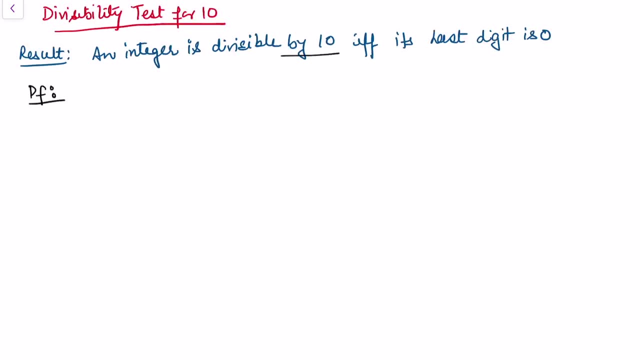 divisibility test. an integer is divisible by 10 if, and only if, its last digit is 0. So, in the similar manner as we have done in the earlier case, simply write n into the decimal format. and here again it is very simple, because 10 is congruent to 0 modulo 10 itself. we are taking, with the respect to the 10, 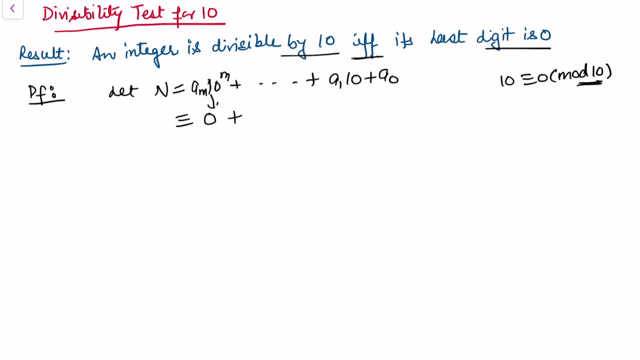 only So each of these quantities are congruent to 0, because they are appearing as a multiple of 10 and the only quantity left is the unit place, that is, a 0 modulo 10.. So we say that 10 divides n, if, and only if, 10 divides a 0, the only possibility for a 0, because we have earlier also said, if we 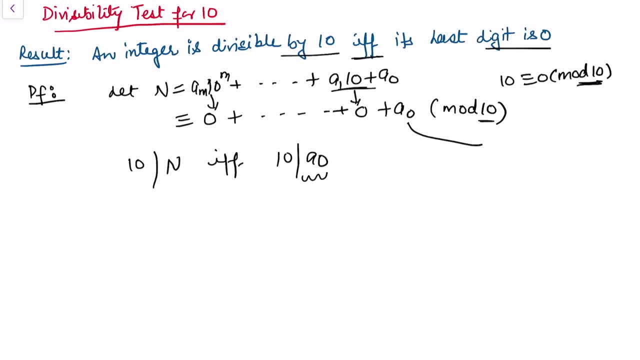 are writing this with respect to base 10. so in n we have written this with respect to base 10.. So each of these ai's here that we have writing these takes a value strictly less than 10 minus 1, or I can say ai's take the value between 0 and 9.. 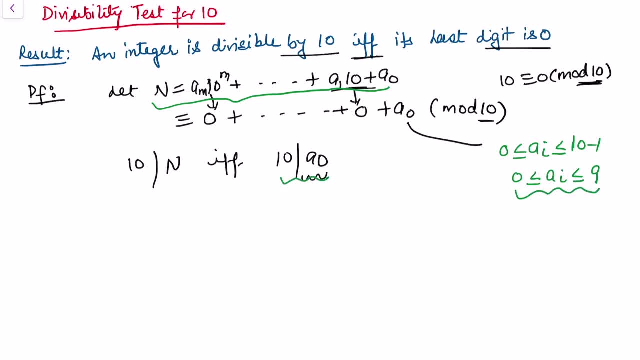 So the only possibility when 10 divide a 0 is that a 0 has to be equal to 0. So only possible choice is a 0 has to be equal to 0, and so 10 divides n if, and only if, 10 divides a 0 or a 0. 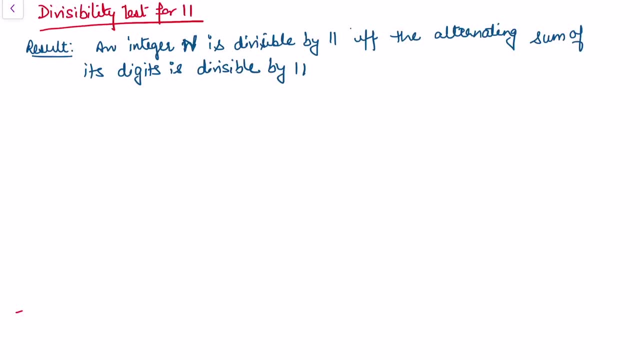 has to be equal to 0.. And lastly, for the divisibility test for 11, an integer capital, n is divisible by 11 if, and only if, the alternating sum of its digit is divisible by 11.. Let's take a look at the divisibility test for 11.. So for the divisibility test for 11, an integer capital, 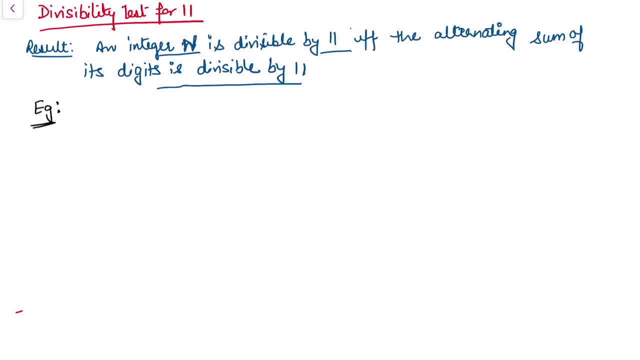 n is divisible by 11, if, and only if, the alternating sum of its digit is divisible by 11.. Let's take an example before we come to the proof of this particular part. If you take capital n, this is equal to 6, 3, 9, 1, 6, 2, 5, 1, 3. and if you take these digits alternatively, starting from this one, so 3. 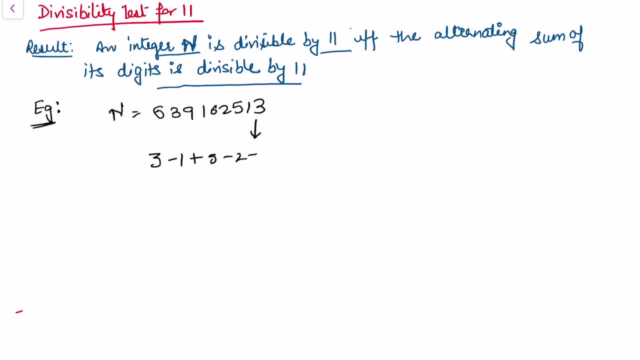 minus 1. then you can take plus 5 minus 2, plus 6 minus 1, plus 9 minus 3 plus 6. this comes out to be 22, and we know that 11 divides 22.. So if this is divisible, we say that the original number 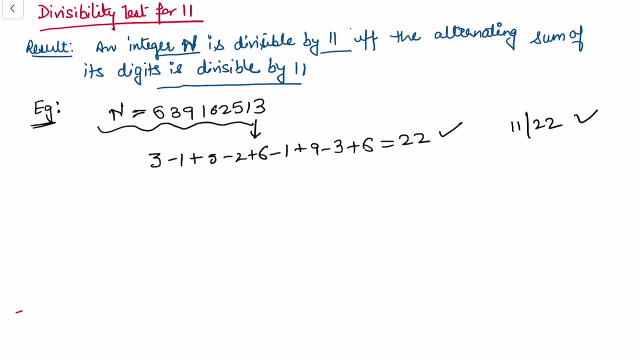 comes out to be 22 and we know that 11 divides 22.. So if this is divisible, we say that the original number comes out to be 22 and we know that capital n is divisible by 11.. Now let's look at the proof of this case Again, in the similar process, I am writing capital n in the base 10. 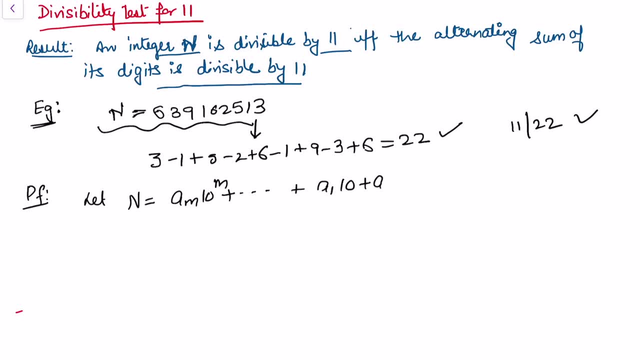 expansion. So here I am writing this as base, 10, and I also know that 10 is congruent to minus 1 modulo 11, because if you take this minus 1 on this side, it will become 11, and 11 divides 11.. 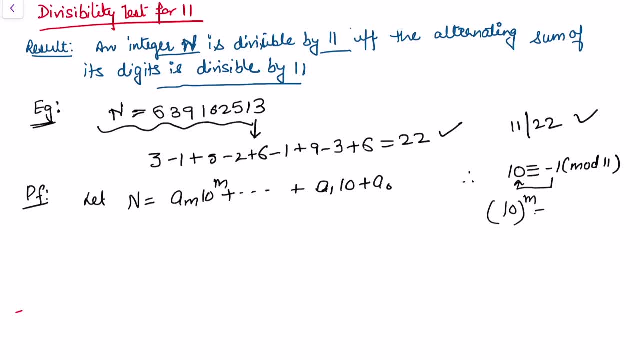 So now, whenever you raise 10 to the power m, this is always congruent to minus 1 to the power m modulo 11.. So if this m is even, I get 10 raised to power m. this is congruent to plus 1, and if this m is odd, I will get 10 to the power m. this is congruent to minus 1 modulo 11.. 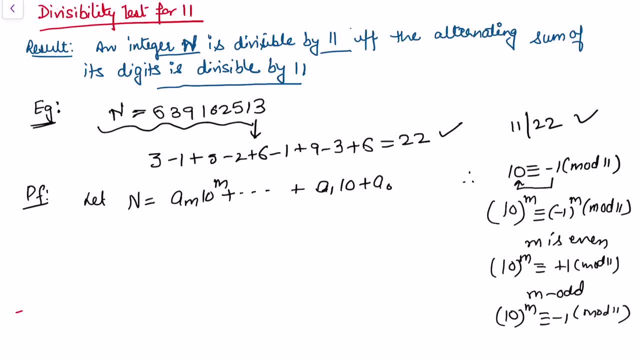 So now, using this fact, let's convert our integer. this is congruent to a naught, will remain a naught, because this is individual unit place digit, and this is not appearing with 10. this 10 to the power 1.. This is odd, so here I have to put minus a1 and then I will have a, so let me to write here a2.